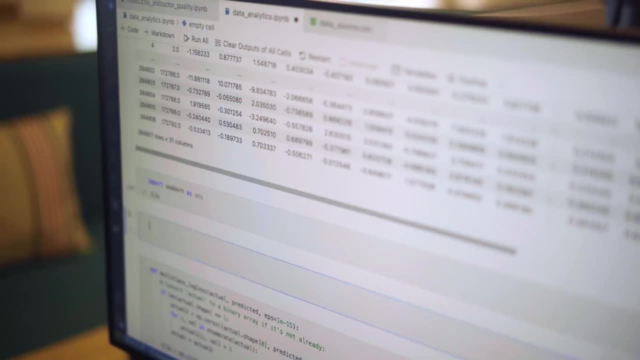 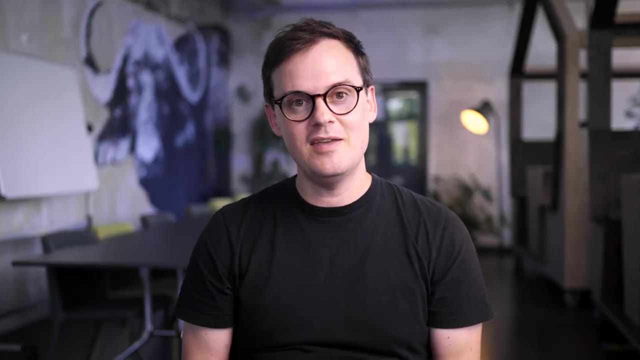 and I'm a senior data scientist at Career Foundry. At Career Foundry, I spend most of my time working with our own company data, But in my spare time there's nothing I love more than working on personal projects, And for those projects I really find it useful to have. 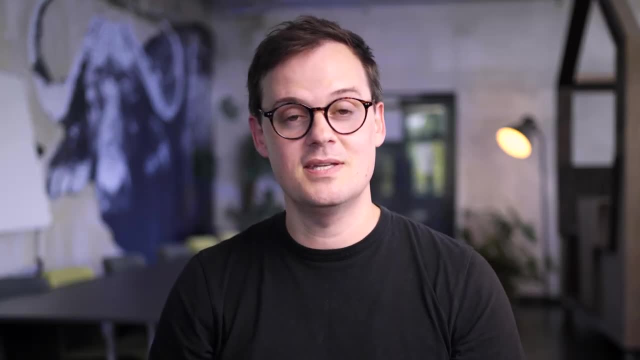 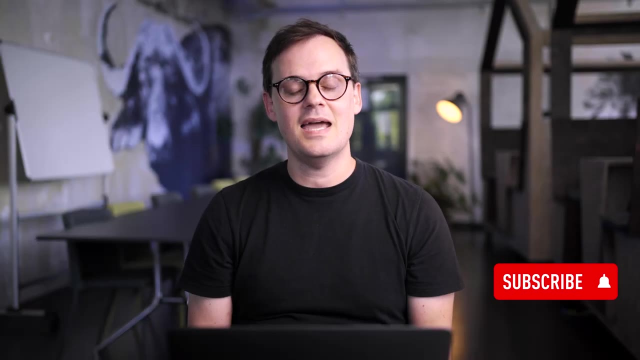 access to free open source data sets. We at Career Foundry have curated 10 places for you to find free data sets coming from a variety of sectors, from e-commerce to environmentalism, and containing a wide variety of types of data, from physics to photography, all of which will 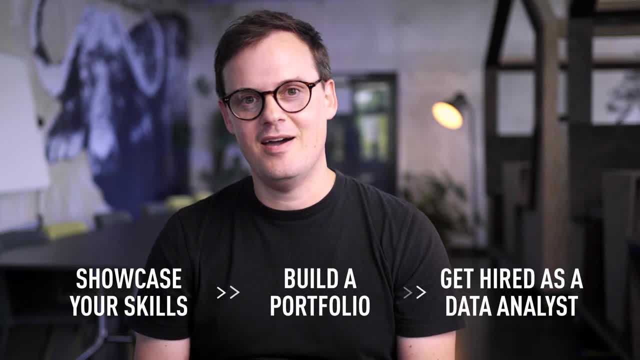 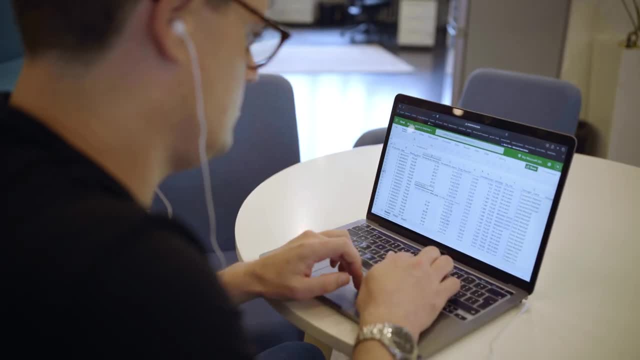 allow you to showcase your skills, build a portfolio and eventually get hired as a data analyst. If you're starting out in data analytics, chances are you're struggling to find access to good data. Maybe you've worked for companies with good data before, but you don't have access to. 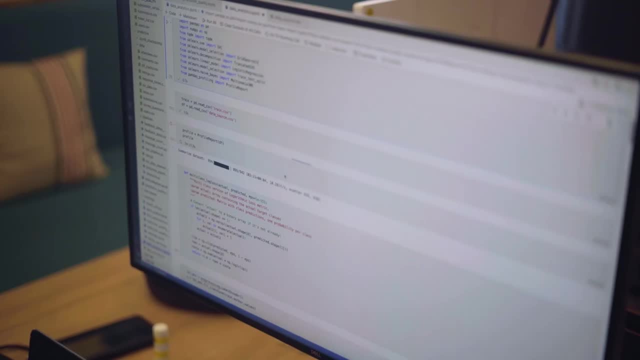 that data anymore. Maybe you haven't worked with APIs before, so you don't know how to pull data from those sources, And maybe your web scraping skills aren't up to score. If you're starting out in data analytics, chances are you're struggling to find access to good data. 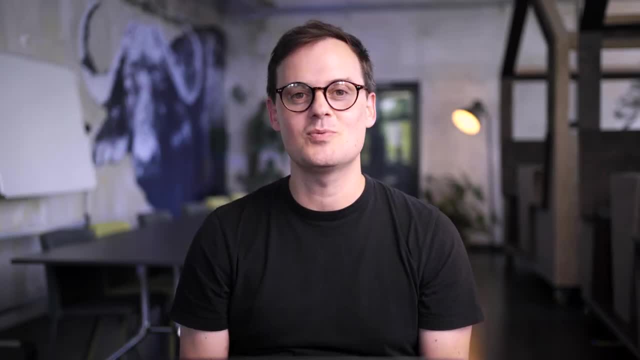 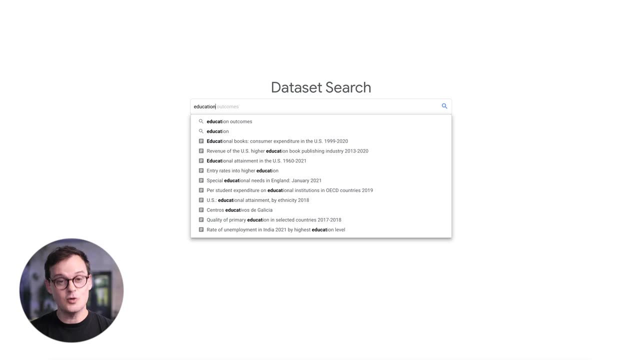 Fortunately, there are tons of free data sets available and we're sharing the top 10 places where you can find those data sets. next, Let's start by looking at the first example now: Google Dataset Search. Launched in 2018,. Google Dataset Search is like Google's search engine. 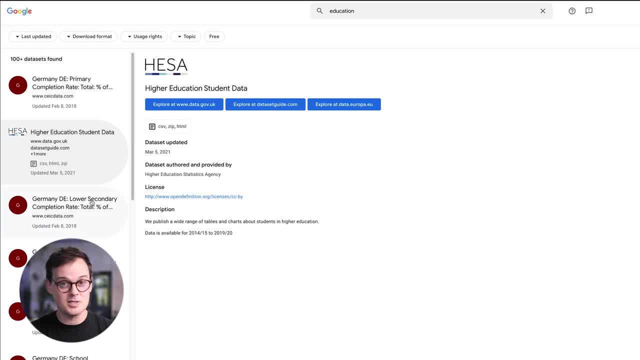 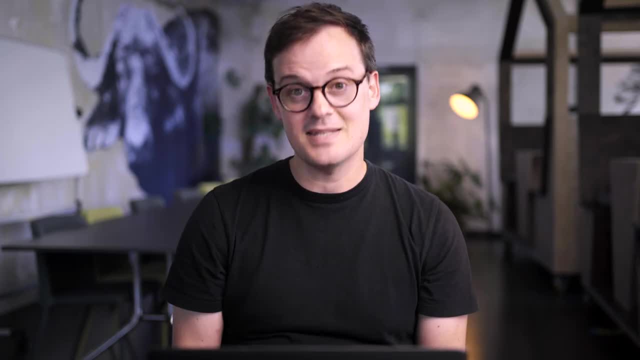 but specifically for data. Google Dataset Search aggregates data from multiple sources, provides a clear summary of what's available, a description of the data, who it's provided by and when it was last updated. It's an excellent place to start Native Python Data Sets. Python has some awesome data. 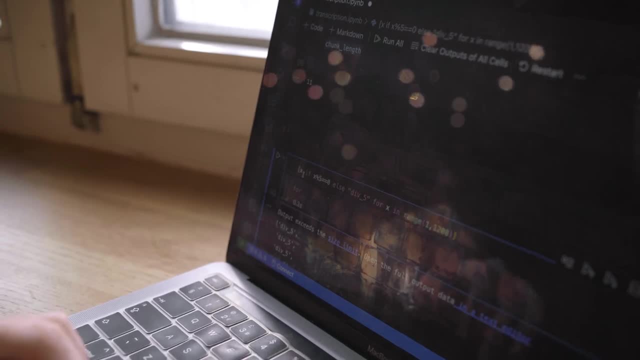 sets that you can use to search for data. For example, if you want to search for data in a search engine, you can use Google Datasets already built into many of the packages commonly used by data analysts and data scientists. Of course, you'll need basic Python skills. 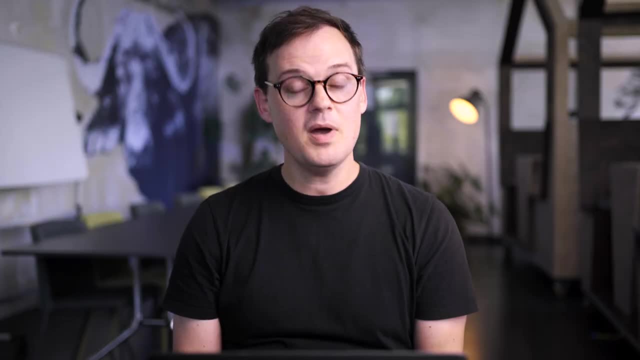 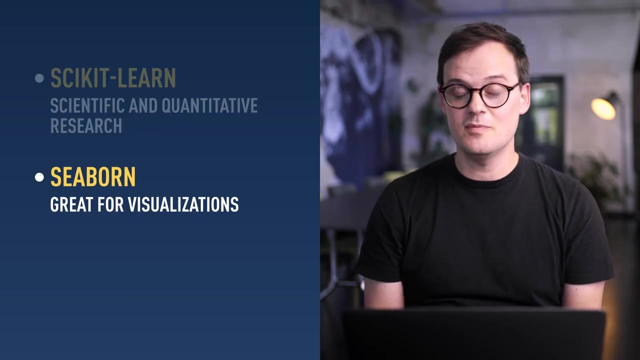 to obtain them, but once you've got those, the possibilities are endless. My three personal recommendations are: Scikit-Learn, a package for doing scientific and quantitative research. Seaborn, a package for doing awesome visualizations. TensorFlow, a package for building and training deep neural networks. 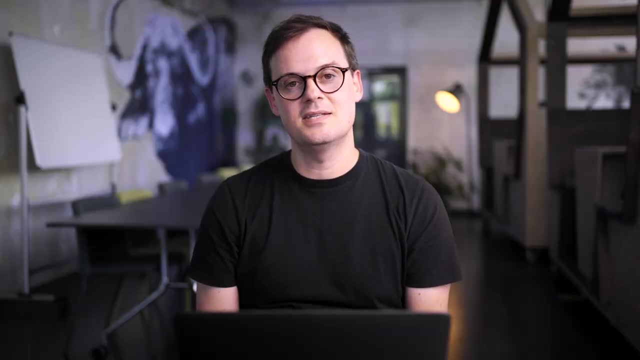 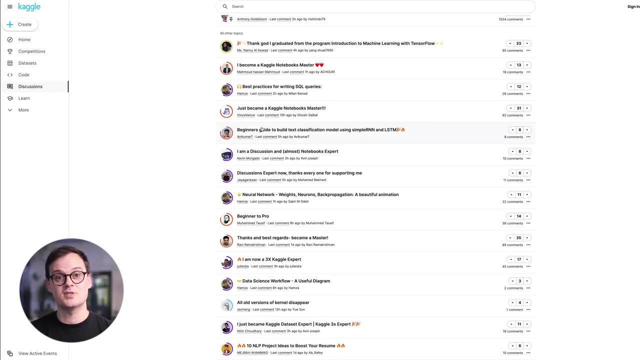 Kaggle. Like Google Dataset Search, Kaggle offers aggregated data sets, but it's a community hub rather than just a search engine. Since its launch in 2010,, it has evolved into a renowned open-source data platform offering online collaboration for 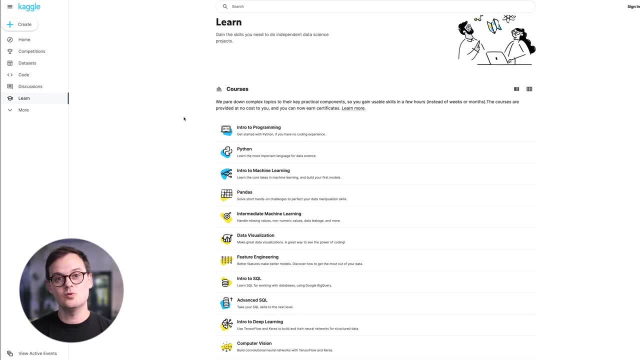 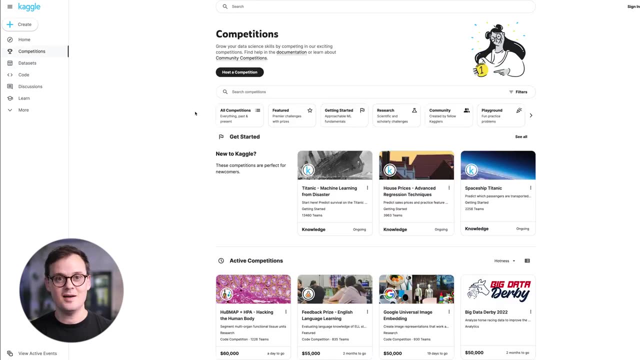 data scientists and data analysts alike, as well as educational tools for teaching data analytics and artificial intelligence. Plus, of course, tons of great data sets covering any problem you can imagine. Plus, you can win tons of money if you solve their problems. But be prepared. 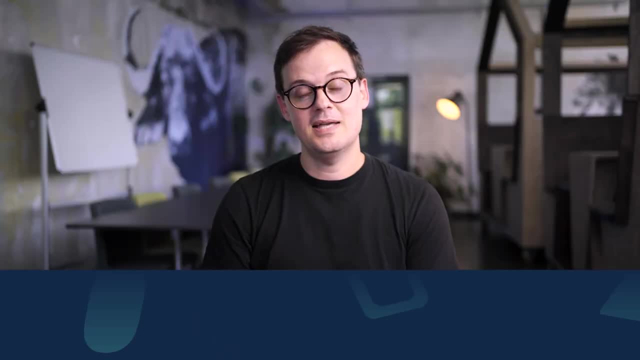 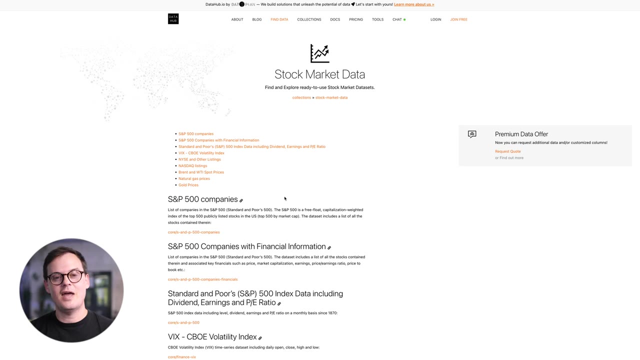 they're not that simple: DataHubio. DataHub has data sets covering a wide variety of topics, ranging from entertainment through to climate change. However, it mainly focuses on areas that can be used to filter, areas like stock market data, property prices, inflation and logistics. 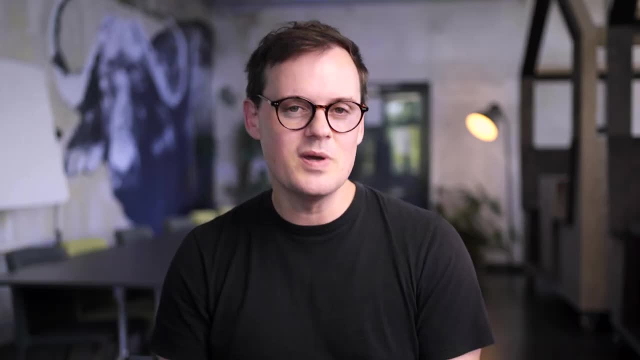 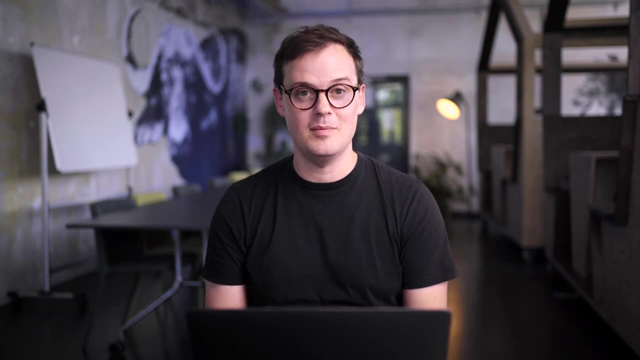 Because most of the data on the portal is updated monthly and, in some cases, daily, you'll always have new data to work with Datagov. In 2015,, the US government made all its data publicly available. With over 200,000 data sets ranging from climate change to crime, there's guaranteed to be something. 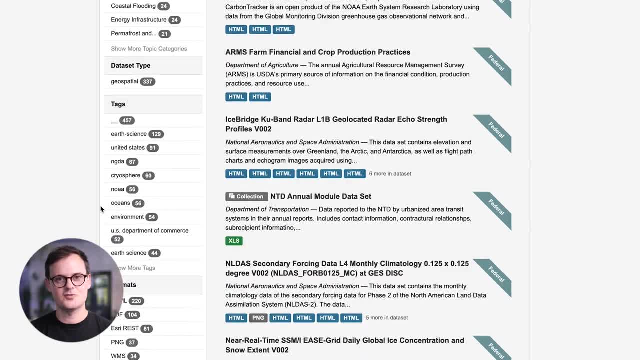 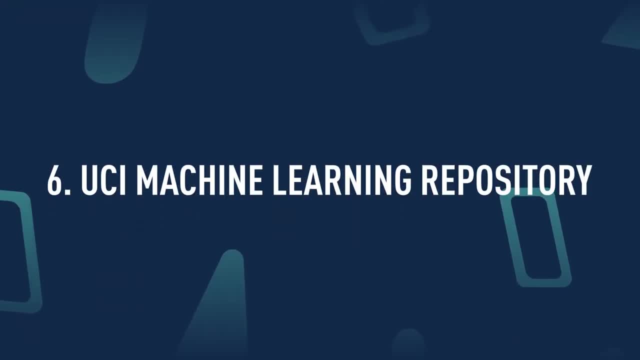 you'll find interesting For a government website. it has some surprisingly user-friendly search features, including the ability to filter by geographical area, type and file format. UCI Machine Learning Repository. If you're looking for something more niche, check out the UCI Machine Learning Repository. 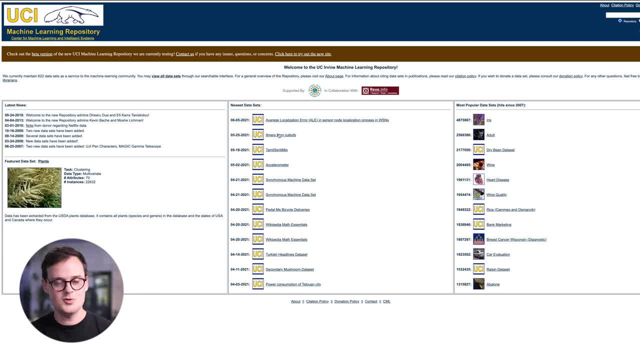 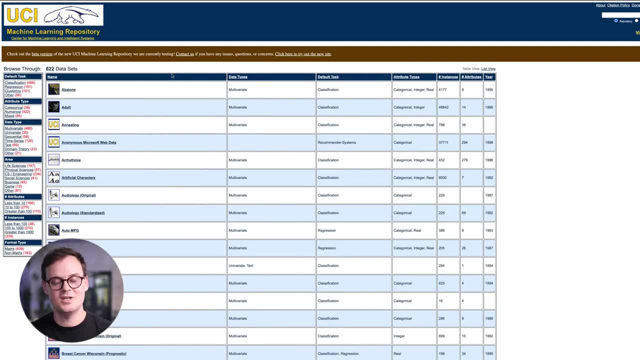 Launched 30 years ago, but don't let the 90s vibe mislead you. the UCI Repository has a strong reputation amongst data scientists and data analysts alike. It's the go-to place for machine learning. data Data sets are clearly categorized by task attribute, data type and area of expertise. 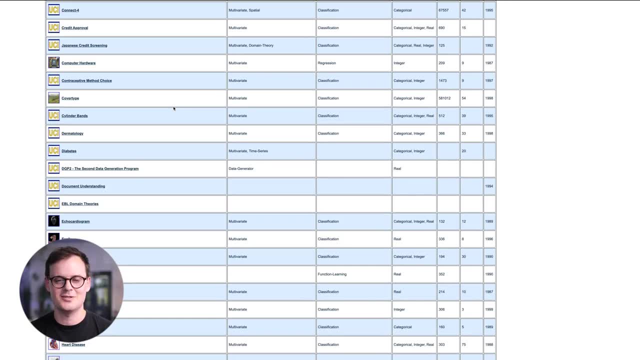 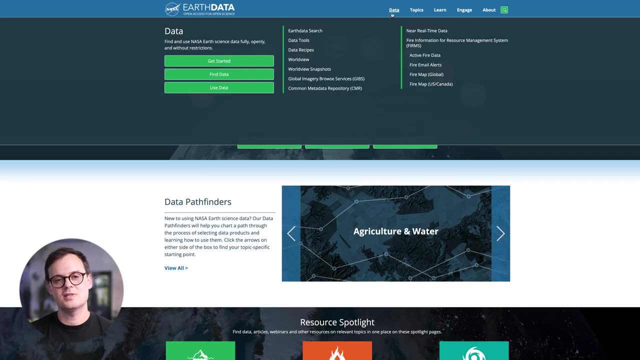 This makes it easy to find something suitable, no matter what sort of project you're working on Earth data. If you think space is awesome- and let's be frank, space is awesome- look no further than the Earth data. Available since 1994,, this repository gives you access to all of NASA's. 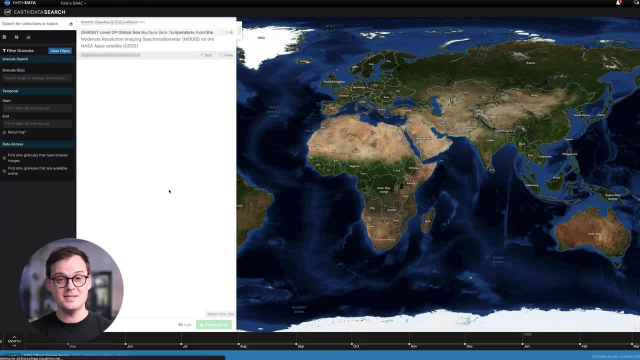 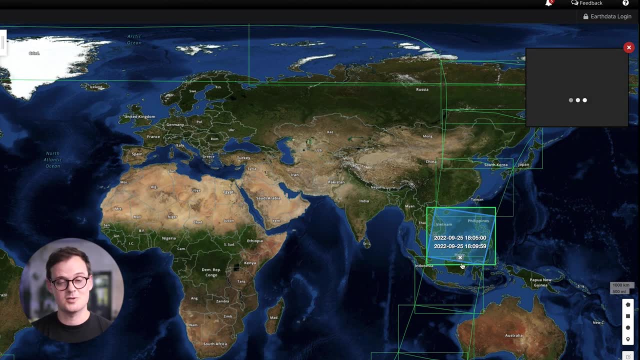 satellite observation data for our little blue planet. There's plenty to peruse, from weather and atmospheric observations through to climate measurements, ocean temperatures, vegetation mapping and much, much more Gapminder. According to the main page of the Gapminder website. 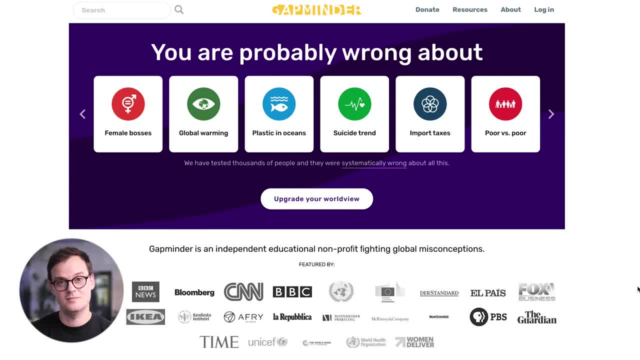 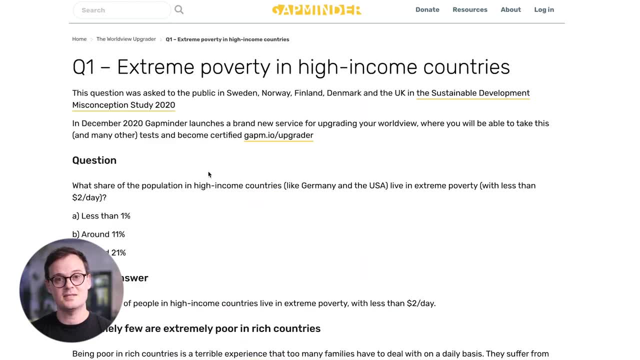 you are probably wrong about your assumptions, across a host of issues ranging from global disasters, plastic in oceans and more. Put together by Hans and Ola Rosling, these data sets are ideal for challenging those assumptions, as well as building awesome data analytic projects.